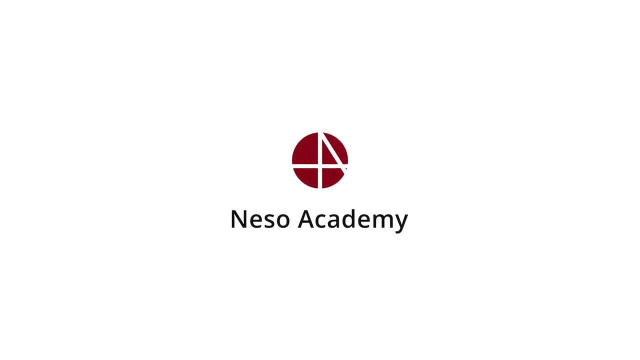 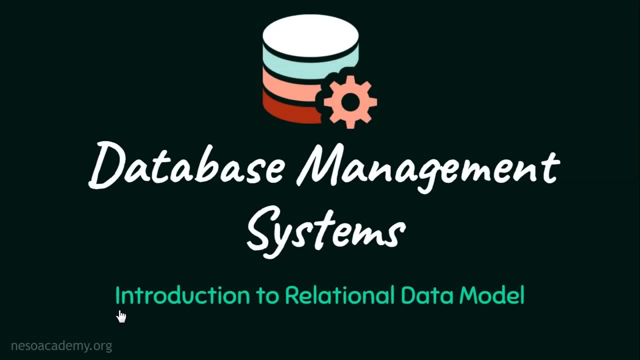 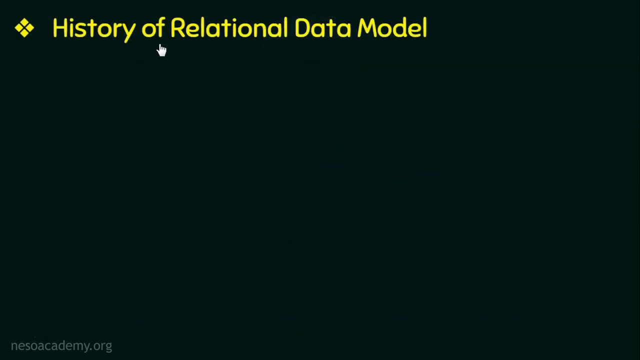 Hello everyone and welcome back to a new chapter in the course of DBMS. In this chapter we are going to learn about relational databases, So in this video we will be looking mainly into the basic introduction to relational data model. First let us look into a brief history of 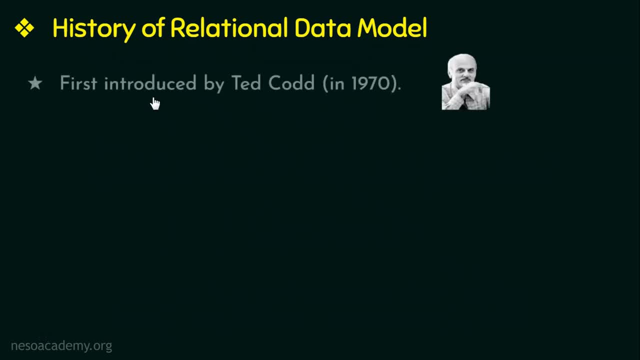 relational data model. The relational data model was first introduced in 1970 by a computer scientist and a mathematician named Edgar Frank Codd, also called as Ted Codd. He was working for IBM when he invented this relational model. In this model, he gave a simple way of storing data. 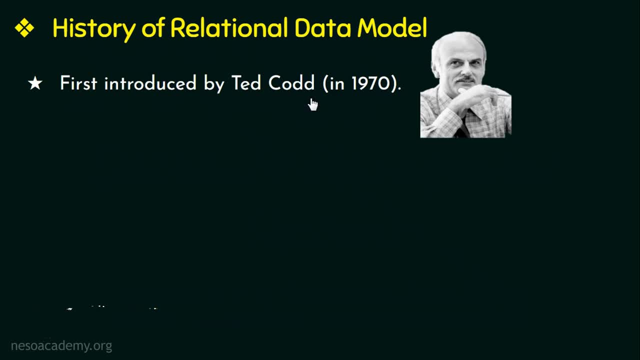 as well as retrieving data via rows and columns in a table. That is, this model was all about organizing data. This contribution of Ted Codd had produced a dramatic or a great change, and, though he has made many other contributions to computer science, this invention of his was his biggest. 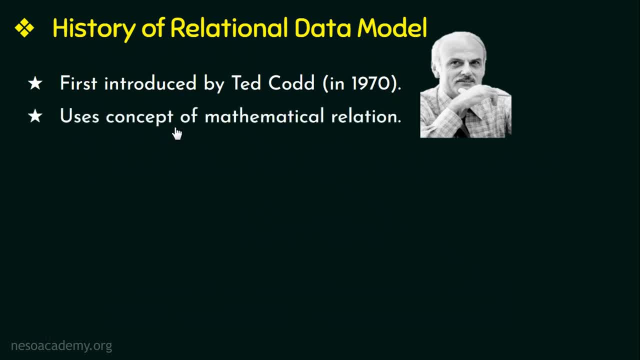 achievement. The relational data model uses the concept of mathematical relations and theoretically it is based on set theory. The first commercial implementations of the relational model was by Oracle, and slowly even IBM started to implement the same, And SQLDS, or Structured Query Language Data System, was IBM's first commercial relational database management system. The current popular 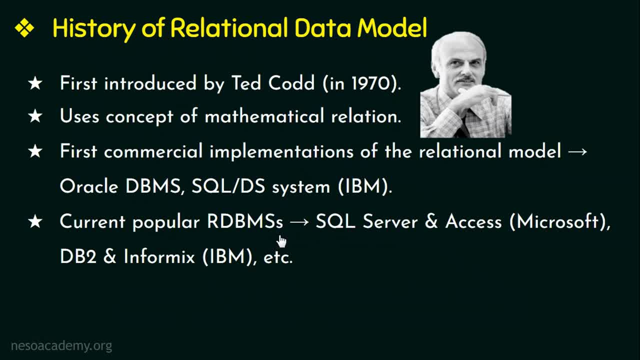 RDBMS, or relational database management systems, are the SQL Server and Access from Microsoft, DB2 and Informix from IBM, etc. And SQL query language became the standard language for these commercial RDBMS. In the later chapters we will be learning SQL query language in detail. 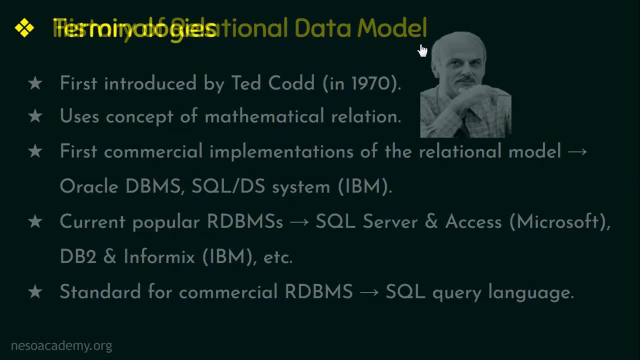 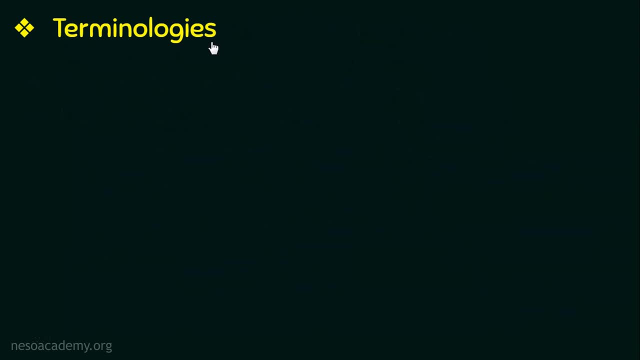 So that is about the history of relational data model. Next, let us learn few terminologies in relation to RDBMS, As I mentioned earlier, a relational database model organizes data in the form of tables, Or in other words, a relational model. 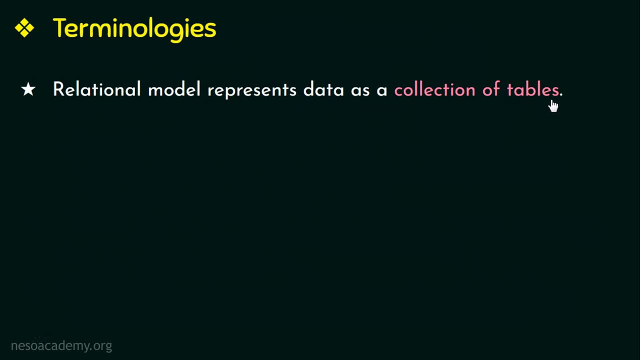 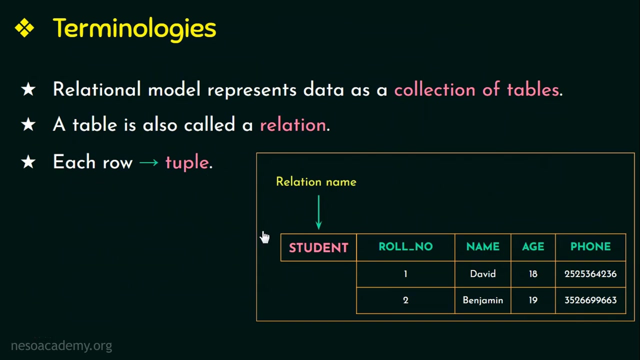 represents data as a collection of tables And here in RDBMS a table is also called a relation. So here I can say a relational model represents data as a collection of relations. In this table that I have taken student is the relation name or the table name, And each row in the table is called a tuple In this. 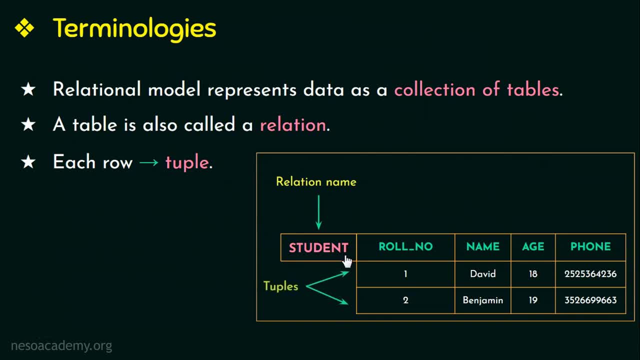 relation, student, we have two tuples or two rows, And each column or the column headers are called as attributes or fields. In this relation, student, we have four attributes of four columns. Hope you have understood these simple terminologies. The next terminology that we are going to learn is: 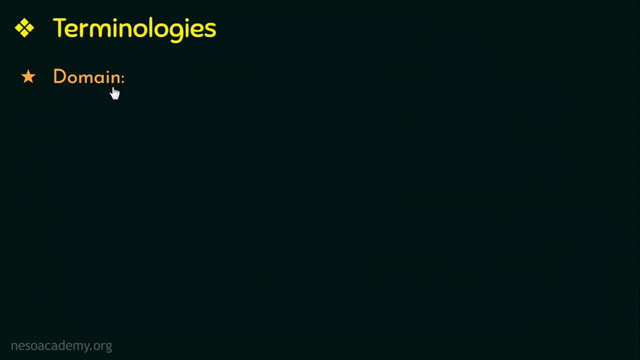 domain. A domain in mathematics is a set of possible values that you can input. So, similarly, in relational database, a domain is a set of values that are allowed for an attribute, And these values should be atomic, That is, each value in that domain. 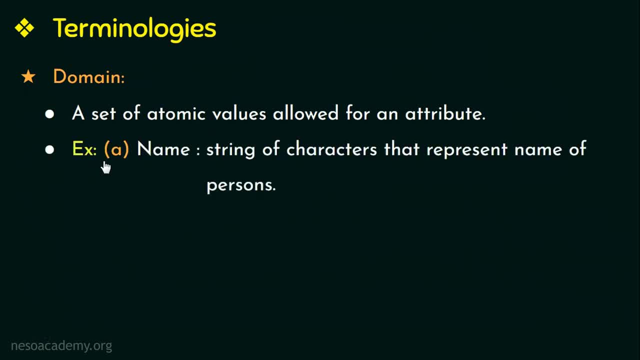 is not divisible further. for example, a set of values for the attribute name should be a string of characters that represent the name of persons, and here the values has to be atomic. another example is domain for the attribute employee ages would be set of atomic values with possible ages of employees. 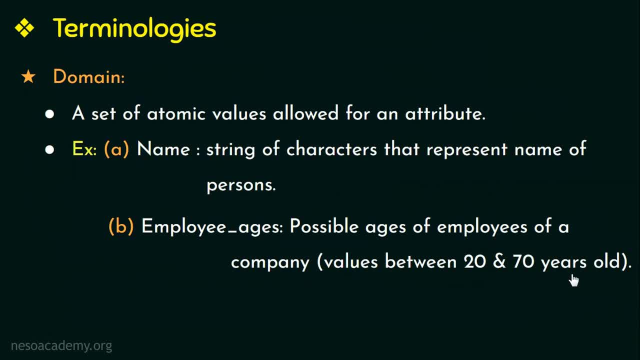 of a company allowed to be between 20 and 70 years old. so hope you understood what a domain is. and domain not only gives a set of values that are allowed for an attribute, it also specifies the data type allowed, like, for example, the age has to be a positive integer. next, what is relation schema? a relation 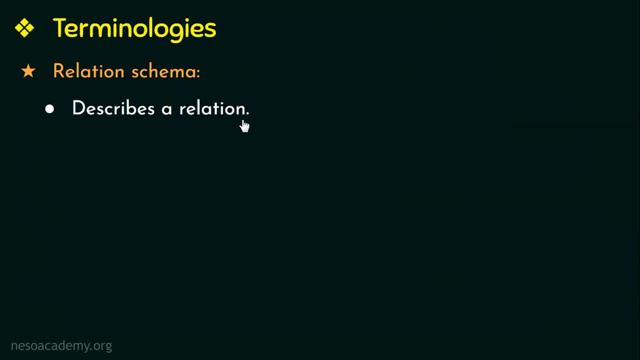 schema is used to describe a relation or a table. a relation schema is made up of a relation name, which is denoted by a capital R, and also it is made up of a list of attributes denoted as a 1, a 2, a 3, a 4, a 5 and a 6. you can also write a relation schema by: 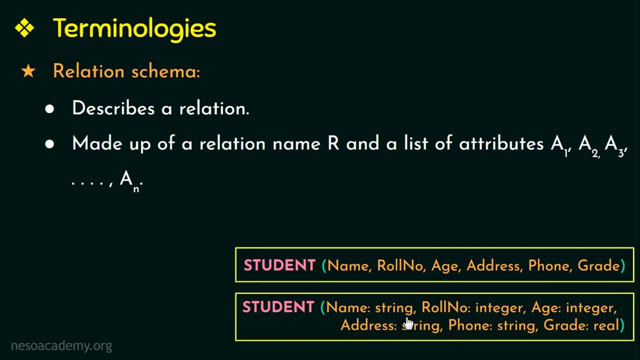 including the data types as given over here, where name has to be a string, role number has to be an integer, and so on. next let us see what is degree or air T of a relation. it is defined as the number of attributes in a relation schema. we just learned what a relation schema is, so in this example of the 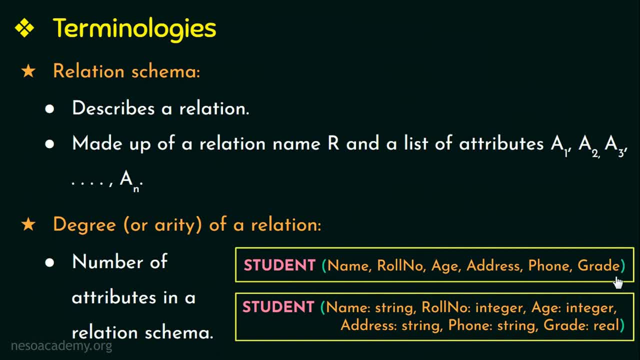 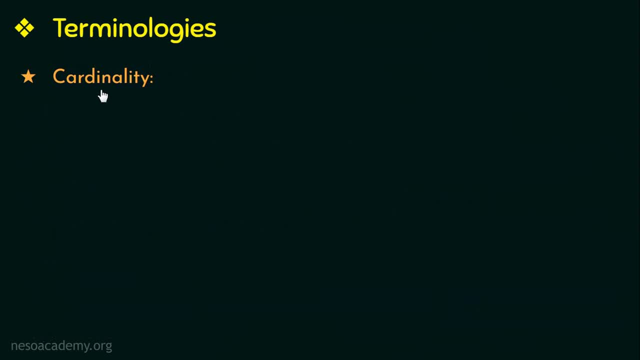 relation schema that we just saw. the number of attributes in a relation schema is 6. therefore, the degree of this relation student is 6. next, what is cardinality? cardinality is the total number of tuples or rows present in a relation. here I've taken a student relation with attributes roll number. 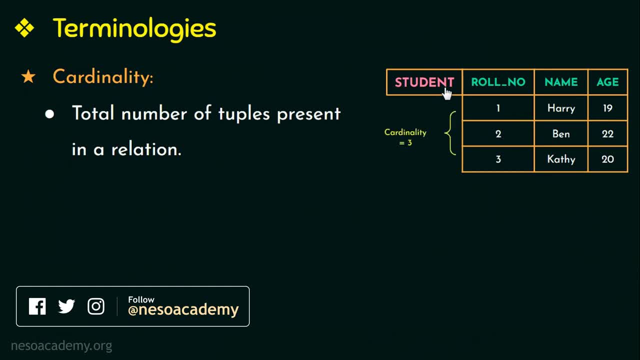 name and age. so the cardinality of this student relation is 3, because there are 3 rows or 3 tuples. the next terminology that we are going to see is relational database schema. a relational database schema is a relational database schema is a set of relation schemas and a set of integrity constraints. that is, if I 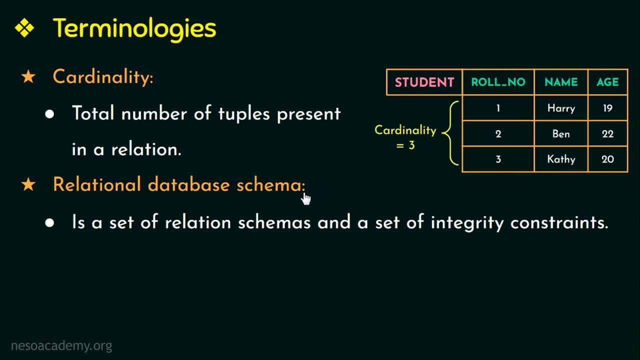 take a company database, the relational database schema of that company would have a collection of relation schemas like the employee relation schema with the employee details, the department relations schema, the project relation schema and so on. so a collection of all these relations schemas, along with the holistic relations schema and interface схemas. preeminent statt all the integrity constraints. 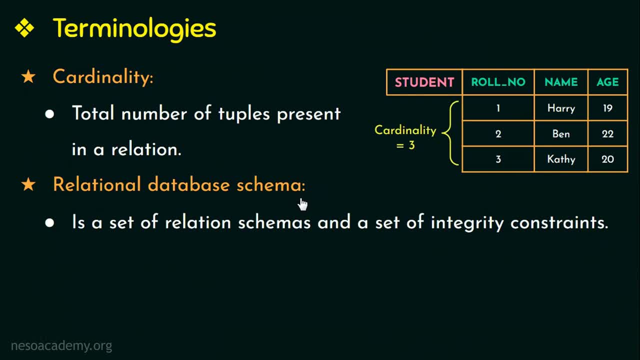 up the relational database schema for a company database. next, what do you mean by a relation state or relation database instance? a relation instance or a relation state is a set of tuples at a given moment of time, like, for example, say, at time t1. this is the set of tuples at that given time. so this is the 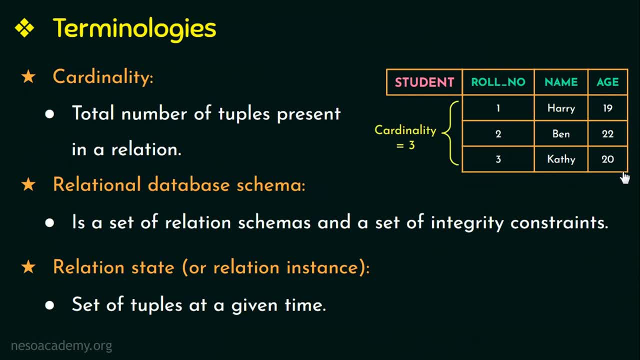 relation state or the relation instance. suppose if I'm updating this relation by deleting this third row, then the set of tuples, say at time t2, would be only these two rows. so that would be the relation instance or the relation state at that given time. so that's it with the terminologies in relation to our DBMS. 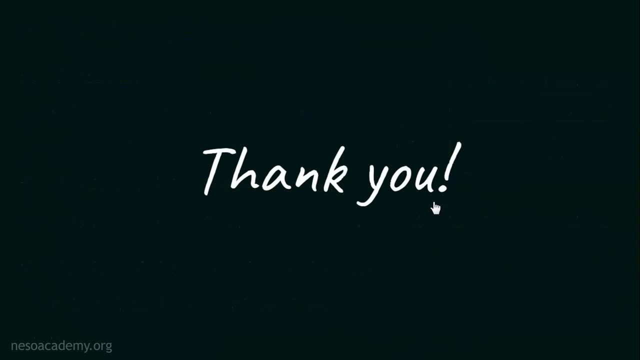 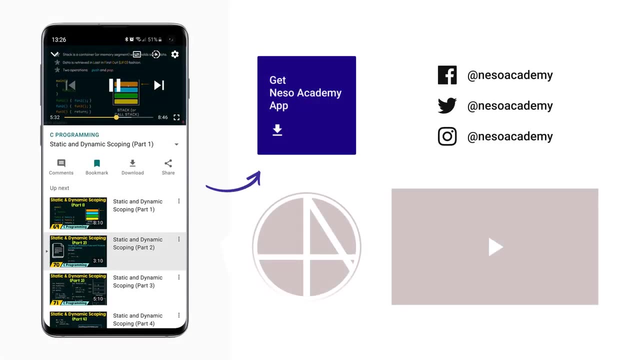 with this we come to the end of this video. hope you have understood all that we discussed in this video. thank you you.